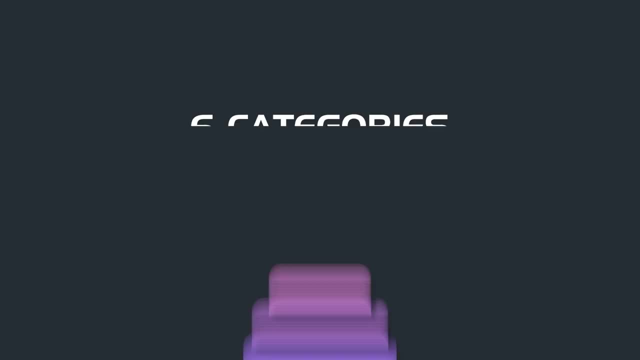 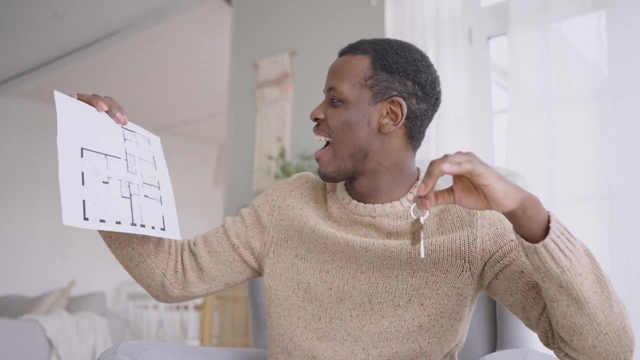 Besides money, there are different reasons why people choose to become hackers. Let's dive into the six categories of different hackers. Black hat hackers can have reasons that range from a desire to secure bragging rights for hacking into a seemingly complex system, tormenting people's. 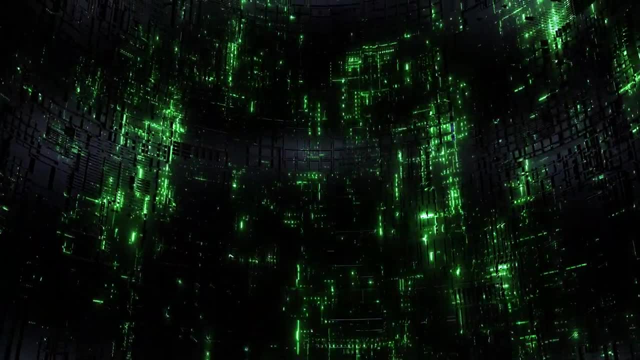 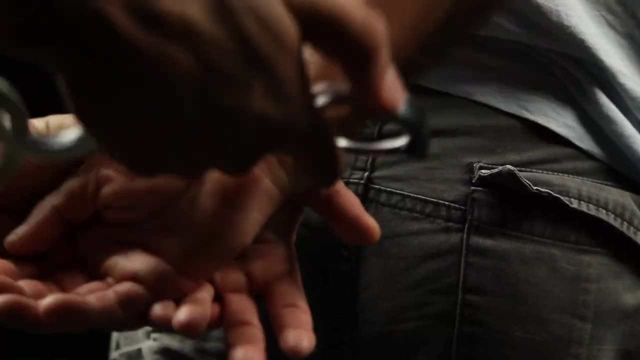 lives for the pleasure of it or simply getting a peek at the map of the world. There are massive volumes of information that public and private establishments would rather not show. Gray hat hackers do what they do for the security of databases, albeit through illegal. 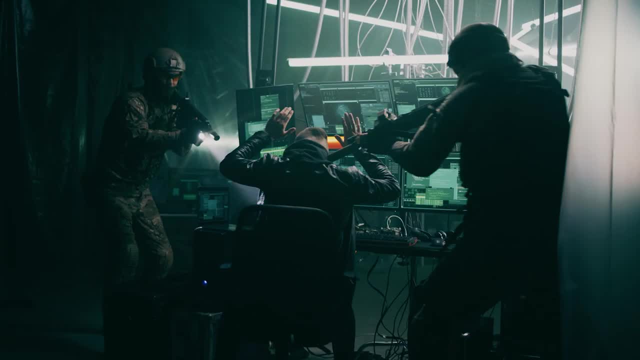 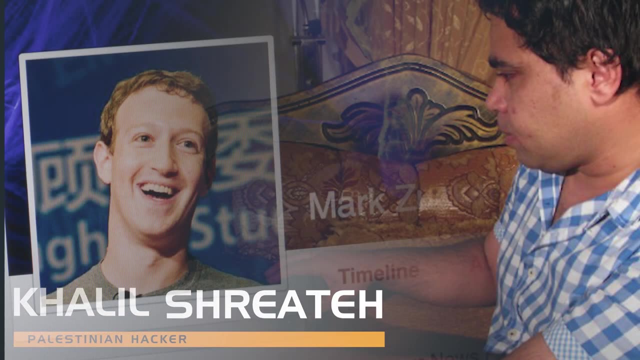 means, and they sort of straddle the line between hacking for ethical reasons and doing it in an entirely wrong way. An example is this Palestinian guy, Khalil Shreti, who hacked and posted on Zuckerberg's Facebook account in 2013.. He had reported a security flaw to the Facebook team. 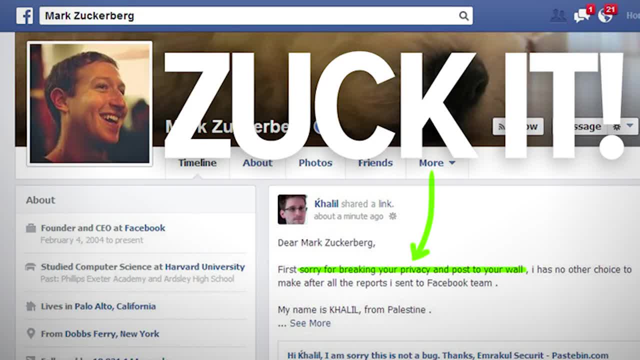 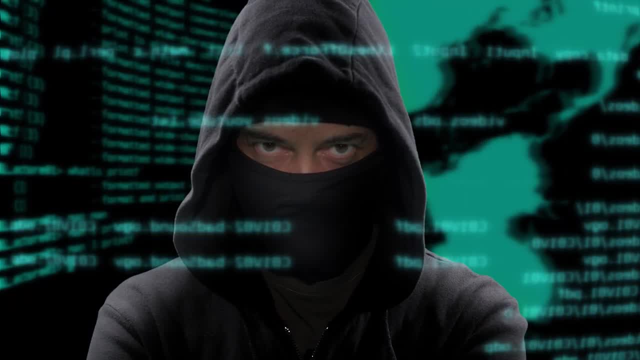 and, when the response was unsatisfactory, decided to take matters into his own hands. White hat hackers are the angels of the law. they are competent and recognizable industry professionals who try to anticipate the works of malicious hackers by spotting system weaknesses before they do, While the actual term was coined. 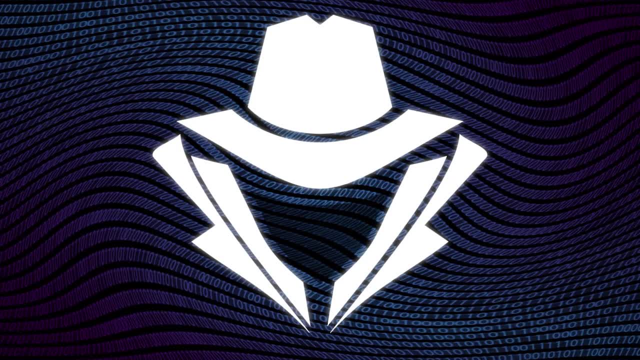 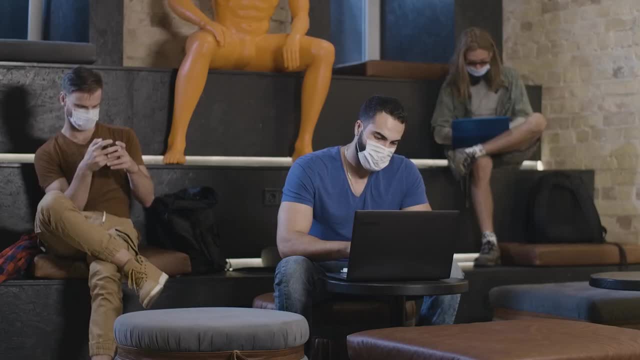 by IBM Vice President John Patrick in 1995,. white hats have been around for almost as long as the idea of hacking itself. In the 1970s, governments created teams to run vulnerability tests on telecommunications and computer networks. These tests are essentially attacks that black hats 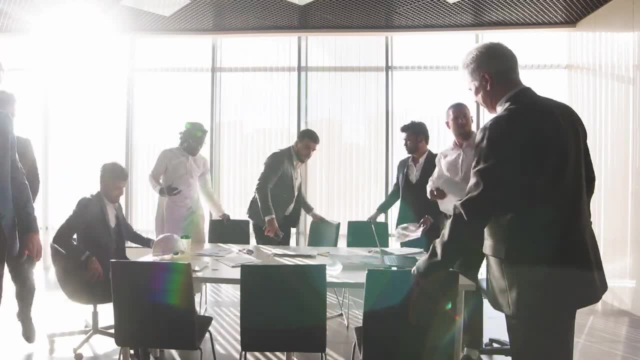 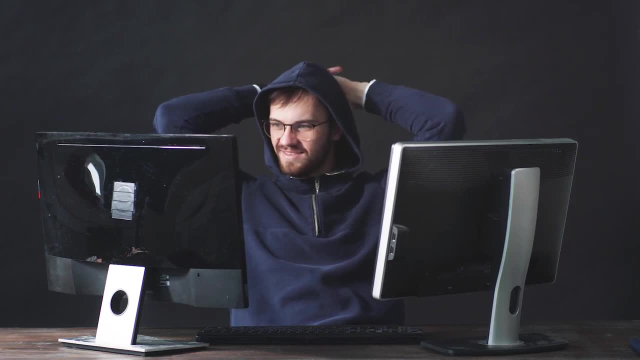 would perform. only this time they are done with the permission and knowledge of the organization. Perks of white hat hacking. Fast over on jail time, obtain recognition as a legitimate hacker and if you're that sort of person, maybe an entire desk to yourself in a gigantic office building. Besides black gray, 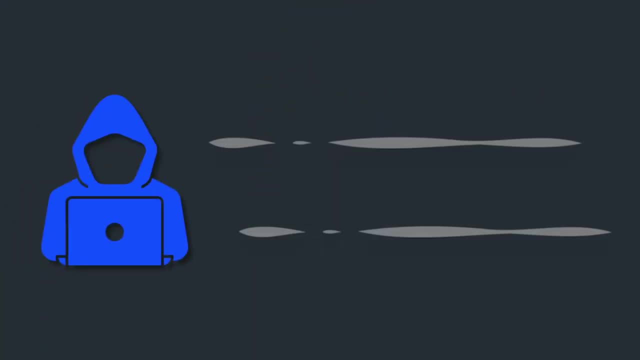 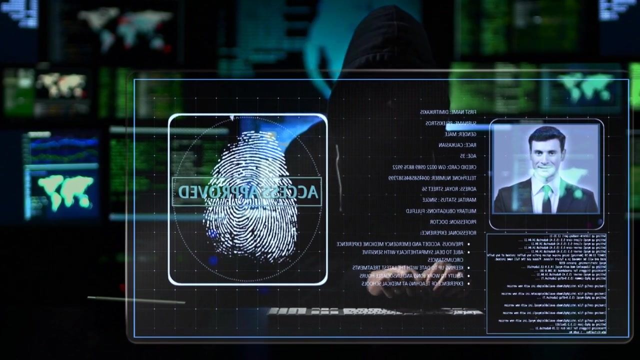 and white. there are even more categories, like blue, red and green hat hackers. Blue hat hackers are divided into two categories. The first category is a group of revenge seekers who use their understanding of computer systems to attack people or organizations they think have offended them. They can obtain access to social media accounts and databases. 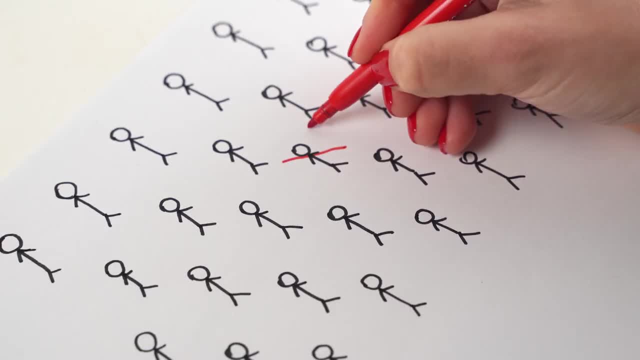 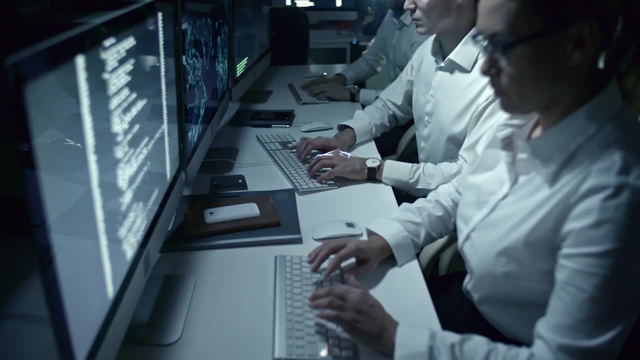 to steal information about their targets and release it to the public. The reason for this is that red hat hackers tend to cause damage to the reputation of their victims. The second category of blue hat hackers are the less vindictive types. They are external security professionals who 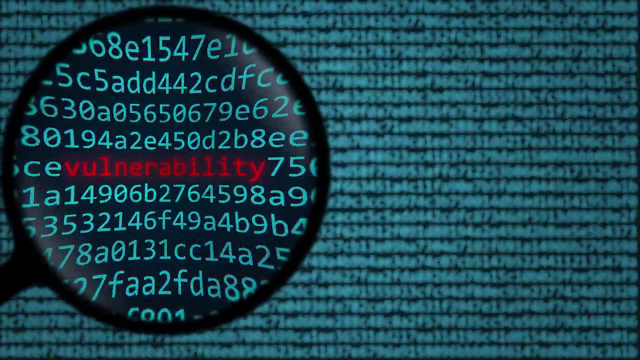 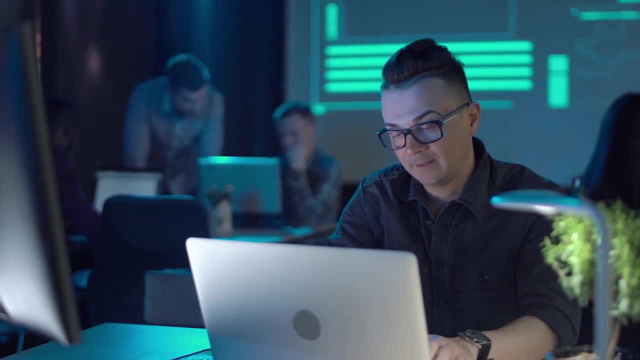 are invited by a company to test software for vulnerabilities before deploying it for use. They do not cause damage to the system, as they merely try to discover potential weaknesses. They may also be hired for collaboration with the company on a periodic basis. Red hat hackers on the other. 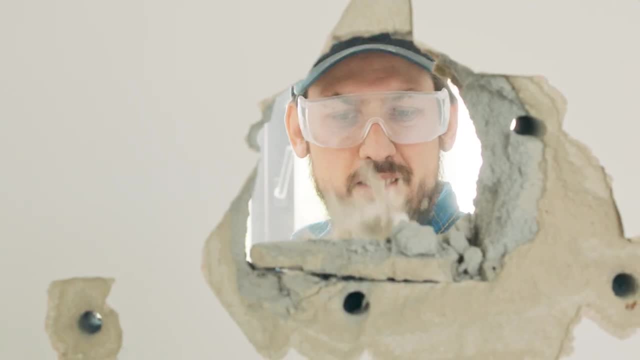 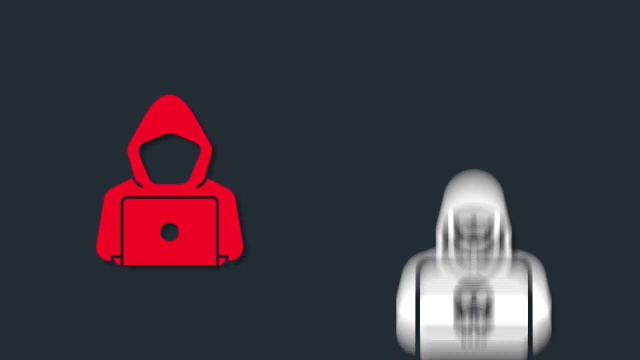 hand, gain popularity for their lack of forgiveness. If you want to mess with the facility, make sure there are no red hatters around, as they tend to go overboard and get caught up in the system. Red hat hackers are similar to white hats in the sense that they have noble reasons for what they. 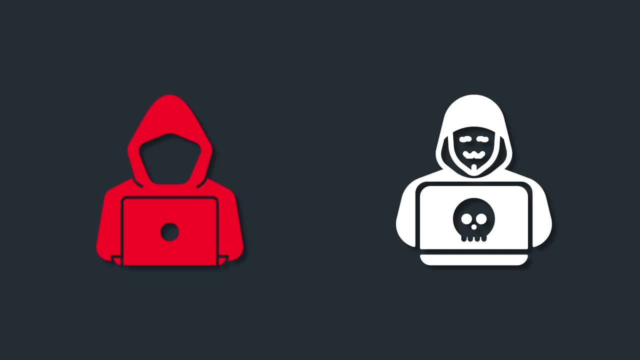 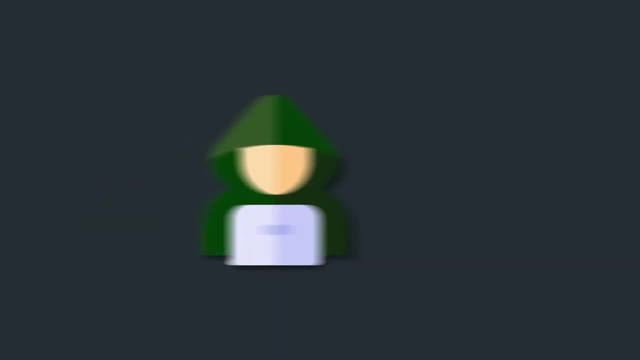 do but diverge in their professional choices. A red hat will typically uncover a black hat hacker, then launch different attacks to cripple their system. They are aggressive and will do ultimate damage to participants they find threatening. Finally, green hat hackers like their name. 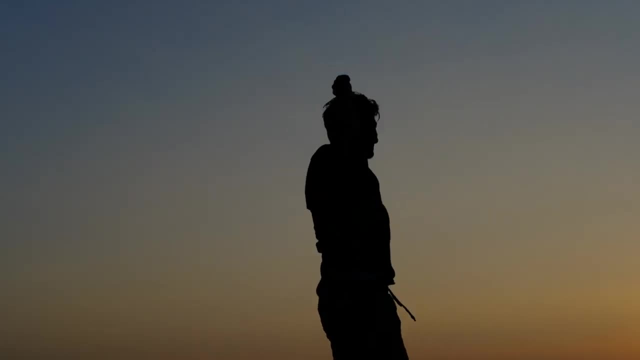 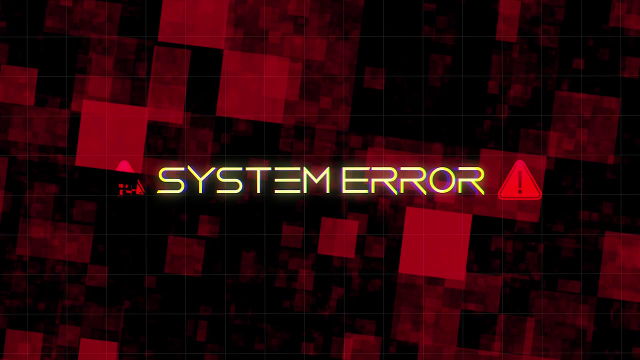 implies are newbies in the world of computer manipulation. They are enthusiastic about hacking, but also do not know enough to properly navigate systems. While experimenting with techniques, they could potentially cause damage without meaning to and with zero knowledge of how to fix it. Blue, red and green classes of hackers can be said to be more flexible. 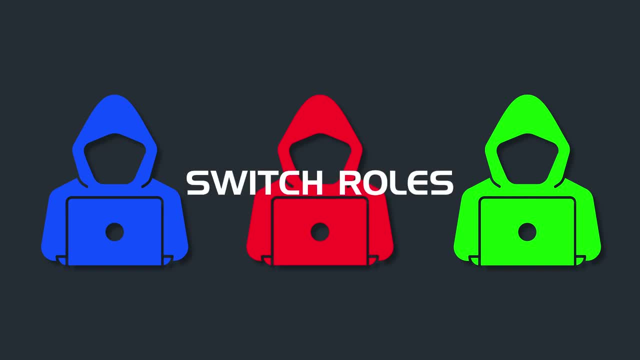 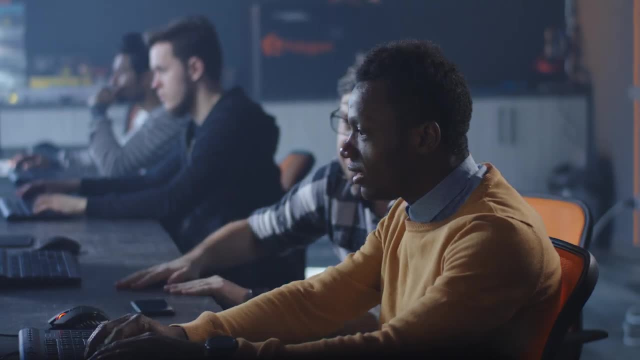 than the first three, as they allow hackers to switch roles depending on their intentions. Since being a black or gray hat hacker is almost certain to get you on the wrong side of the law, we will only discuss white hat or ethical hackers. Why would you become one? 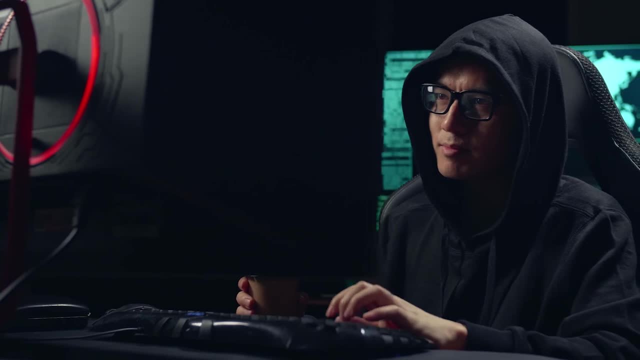 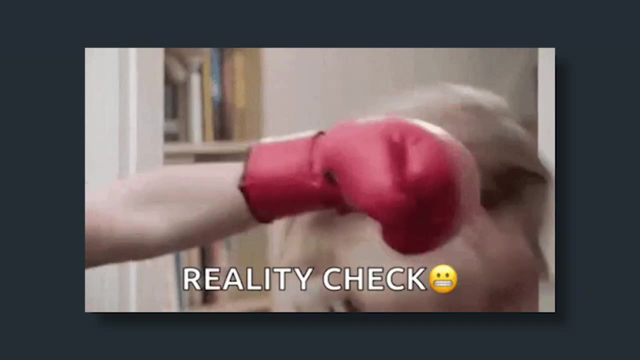 Before deciding to become one, the first thing you need to know is that ethical hackers are not exactly the richest of the pack, so if you're heading into the industry with the belief that you can make a ton of money, reality check: this job might not be for you. On the flip side, 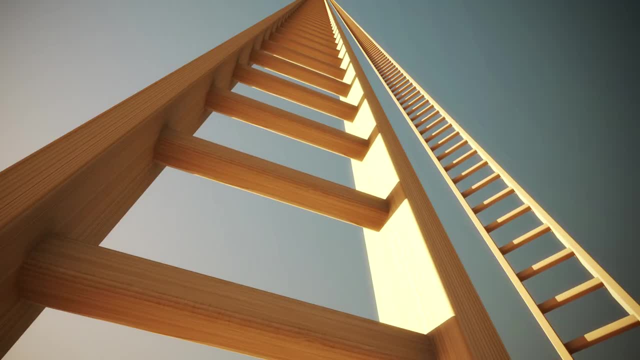 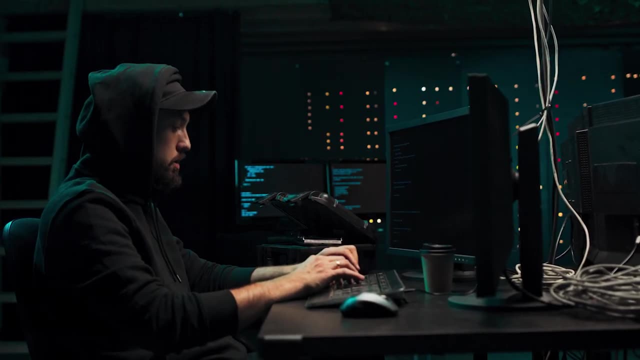 if you intend to practice hacking for the actual professional thrill, you just might land yourself a definitive and highly rewarding career path. White hat hackers are consistently in demand because of the activities of bad actors on protected systems. They earn an annual salary that is north of $80 to $100,000. But beyond that, 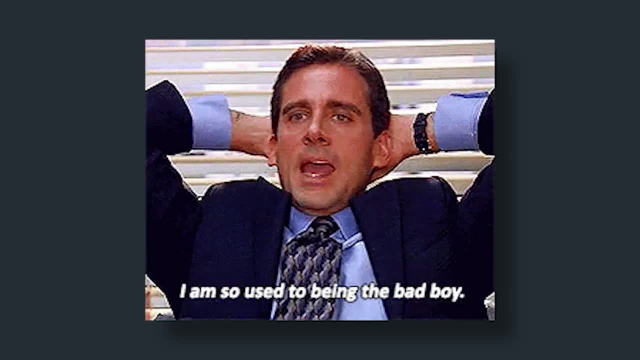 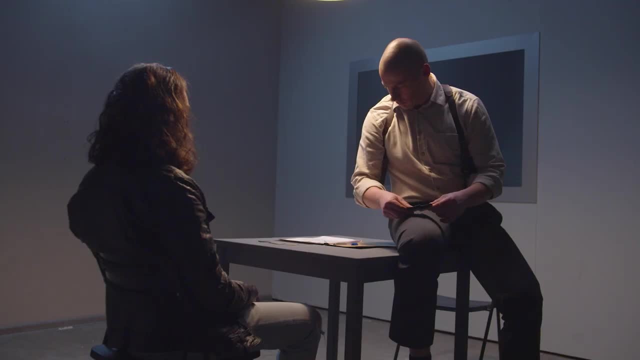 get to be the bad guys without being the bad guys. Think of it this way: you get to run attacks and find vulnerabilities to your heart's content, develop fixes and then get paid without needing to send a ton of nasty messages or hook the FBI up on your internet footprints. Also, you get access. 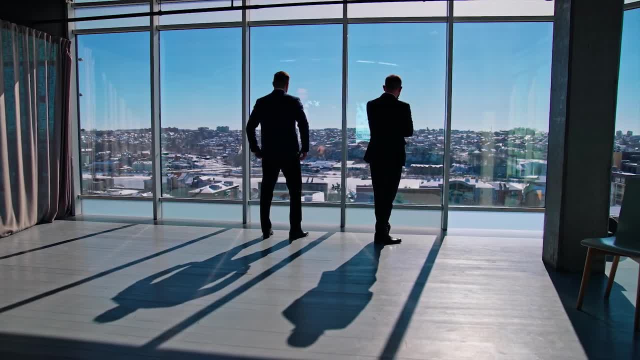 to better hacking training and resources than black hat hackers. If you are a black hat hacker, you might want to learn more about hacking. Most large companies you will work with will already have a budget in place for network security. They will naturally invest this in training their experts. 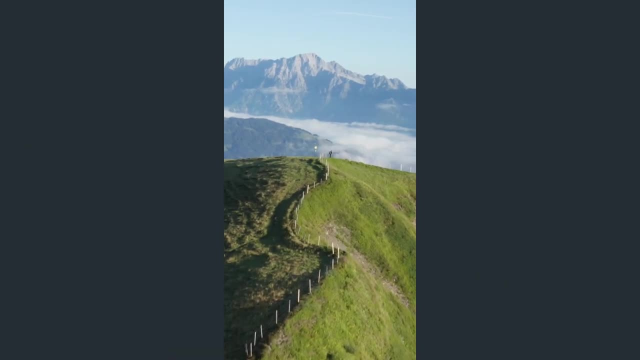 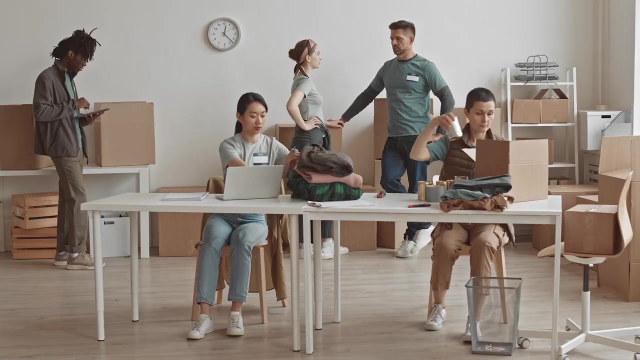 in new techniques, translating to a broader learning horizon than a self-funded actor would normally get. What are the risks? Still, white hat hackers do not always have it smooth. Because organizations have to preserve expensive equipment from damage, hackers have to tiptoe around them in. 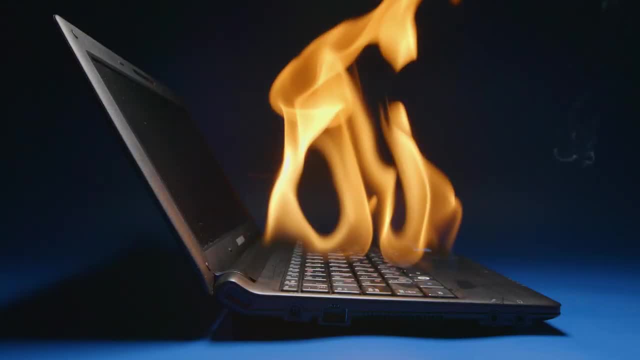 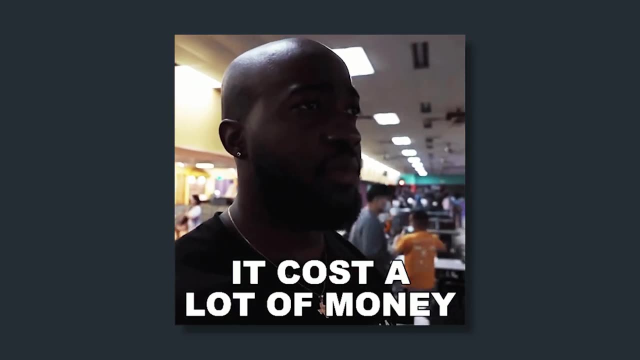 penetration tests, There is a limit to how aggressive they can be, as damage to systems could lead to financial loss. On top of this, simulations do not always represent the real world. Equipment costs will typically prevent companies from providing additional facilities for test purposes, forcing hackers to assume. 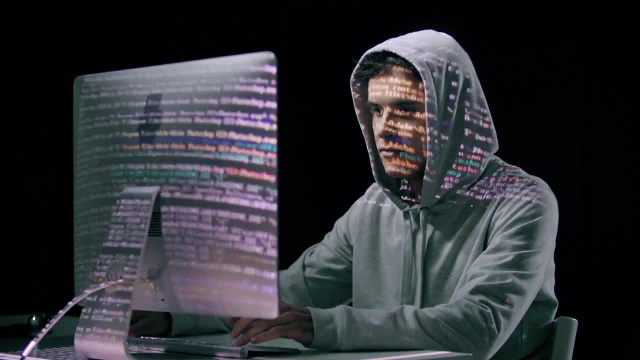 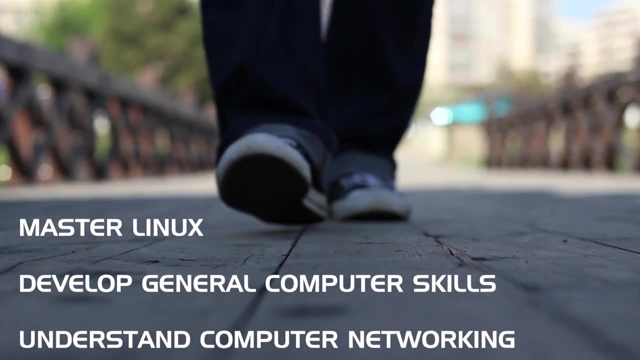 that malicious actors will follow the same pattern as their bare minimum attacks. What needs to be done to become one yourself? Now that you know the benefits and the risks of white hat hacking, let's talk about the things you need to do, step by step, to become one. You can find all the links. 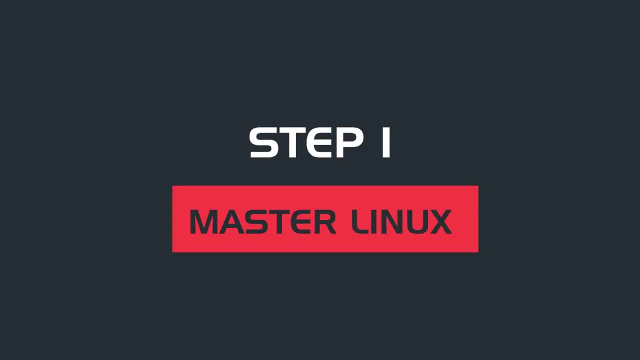 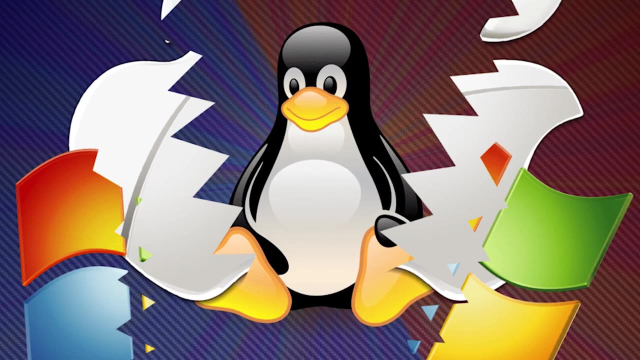 to the tools that are mentioned in the video in the description Master Linux. Are you using Windows or Mac OS at the moment? Stop it right away. The Linux OS is one of the most secure operating systems in the world today. It is a favorite among security. 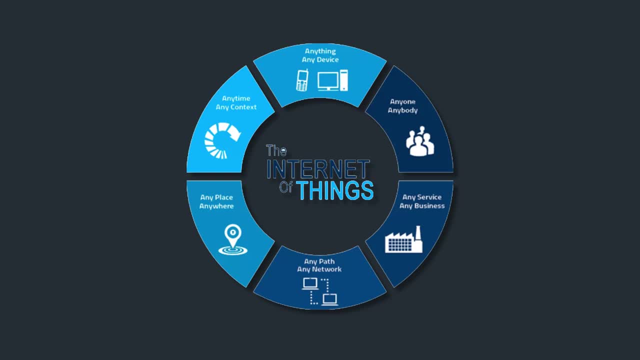 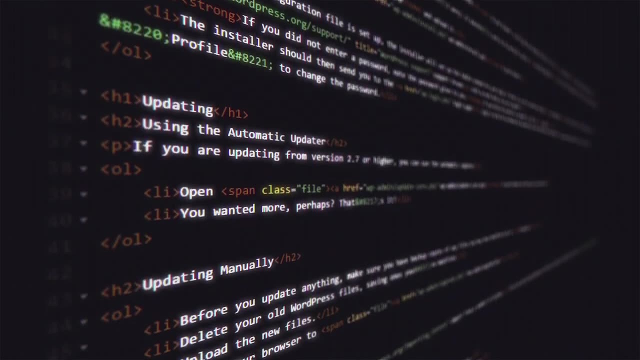 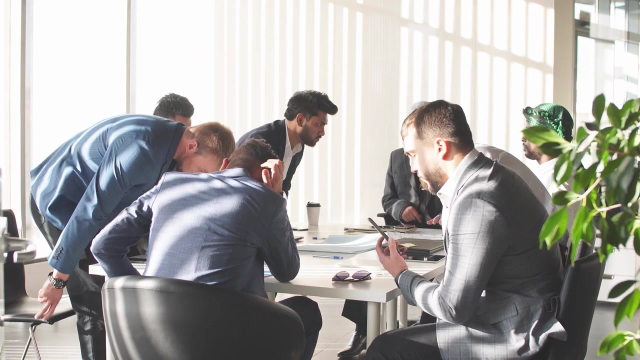 experts and is leveraged in the development of multiple internet-based devices. Hackers are often advised to understand Linux because it also runs on open source code, which individuals and corporations can manipulate to their tastes. Added to these is its transparent nature, which is one of the biggest wins over Windows' ecosystem and a deciding factor for companies. 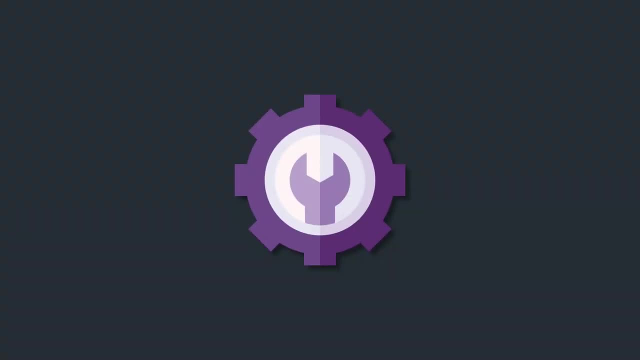 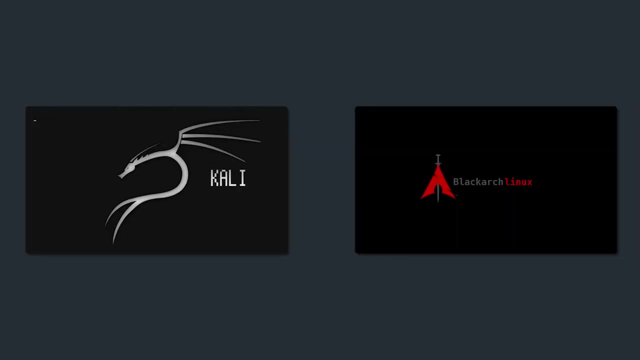 that prioritize control. A lot of the tools that you will use for hacking, such as Python and Bash, are also designed for this system, making it an inevitable success anyway. Kali Linux and BlackArch are currently some of the most common distributions for use at the moment. They incorporate numerous hacking tools- more than 2,300 in the case of 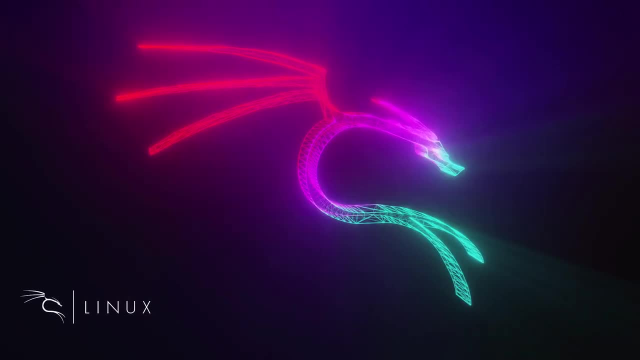 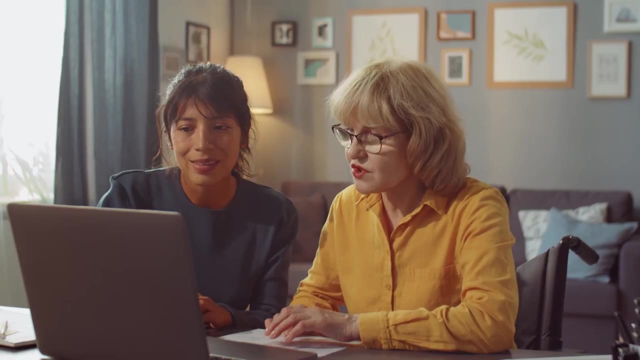 BlackArch. Kali Linux is both a fan favorite and the most stable of the pair due to its existence over a longer period. Develop General Computer Skills. Another thing you cannot do without is the possession of computer skills. This is the most elementary bit of a white- in fact any hacker's- professional life. You need to be. 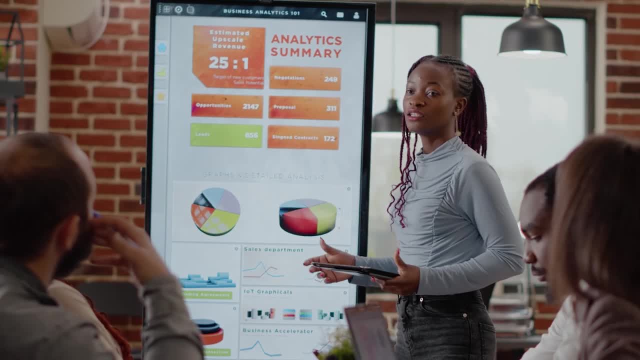 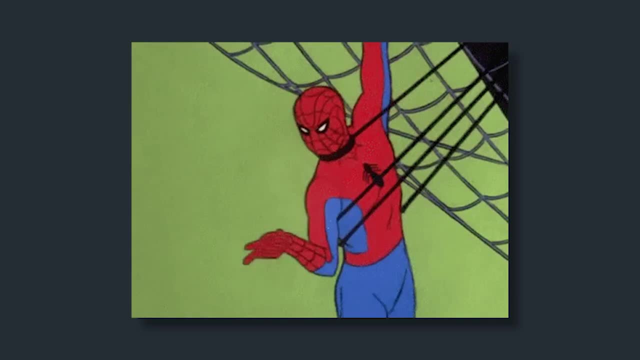 competent in file management, data processing, spreadsheets, presentations, etc. To evolve, become a fully-rounded hacker. Train yourself in the use of Microsoft applications, database management, social media, web enterprise systems and all the other major stuff that. 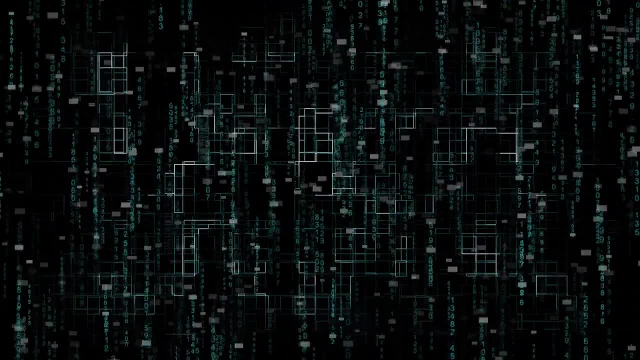 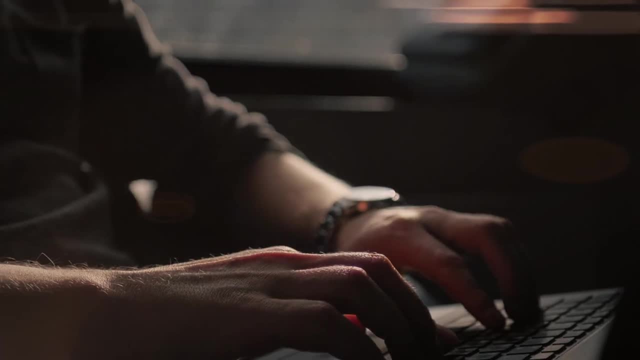 will prove critical to your role. Understand Computer Networking. A computer network is essentially the interplay of multiple host devices which extend across data-transmitted pathways. To become an ethical hacker, it is important to acquire skills in subnetting, supernetting, DHCP and a variety of others. 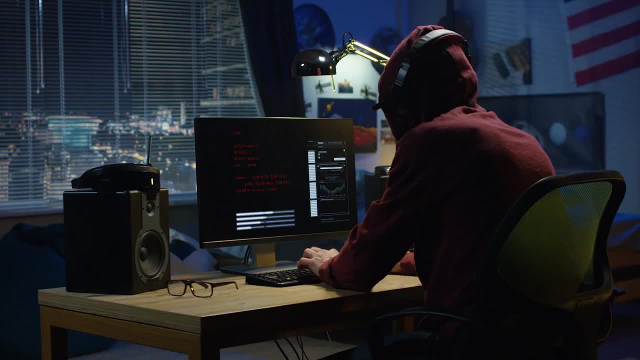 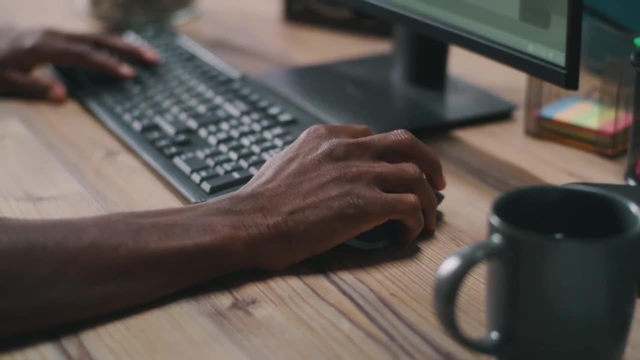 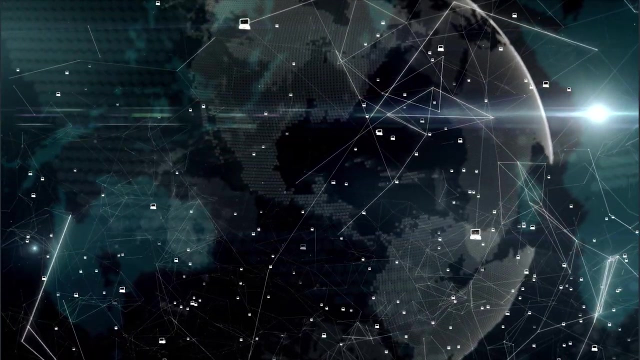 These enable you to look deeply into how network components operate and the vulnerabilities that exist in their structure. Once you are familiar with that area, you can then proceed to outline the most appropriate responses to specific threats. It is equally important to understand that the field of computer networking is quite broad and will require you to take learning one. 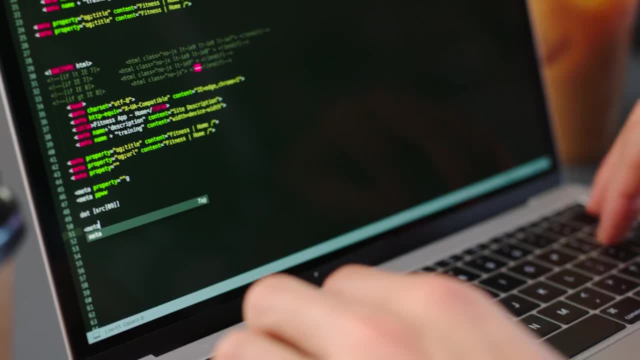 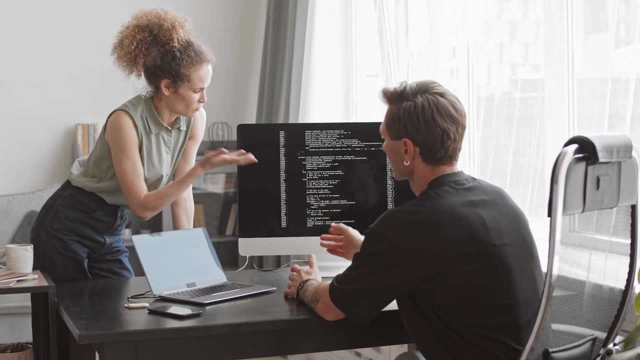 step at a time, Learn Computer Programming. Programming is basically the construction of commands in a language that the computer understands and can execute with. It is one of the most important pillars of an ethical hacker's career and is best learned with practice. There are different programming languages you can use as an ethical hacker, but the most recommended one would be a computer-based network. If you are an ethical hacker, you can use both out-of-the-box and out-of-the-box networks to create a network of different types of networks where you can use your computer to work with the needs of other. 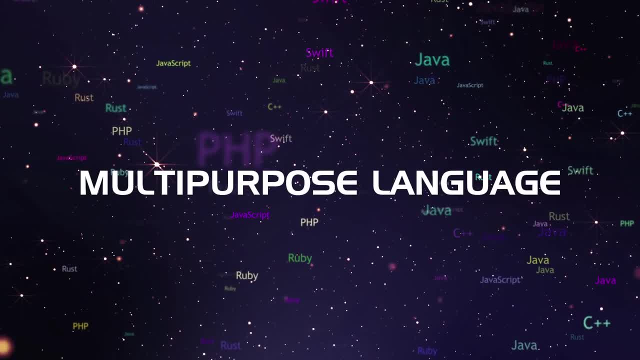 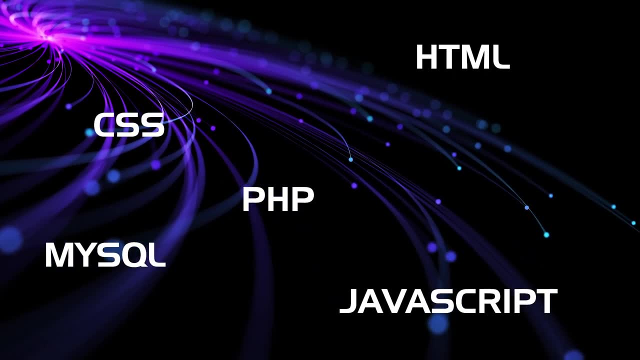 people Learning Computer Programming. recommended one would be a multi-purpose language to help you automate several of your deliverables. There are web programming languages like HTML, CSS, PHP, MySQL and JavaScript. There are also others like C and Python. All of these are pretty straightforward to learn and will reflect in the 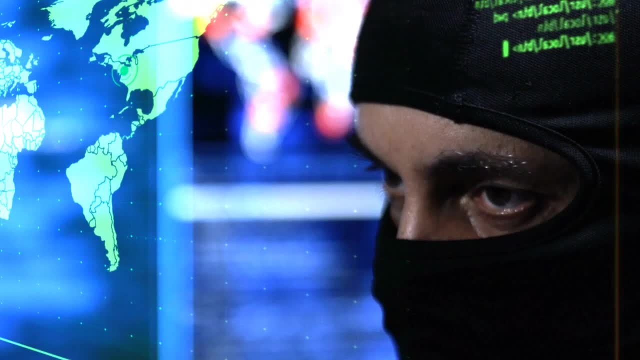 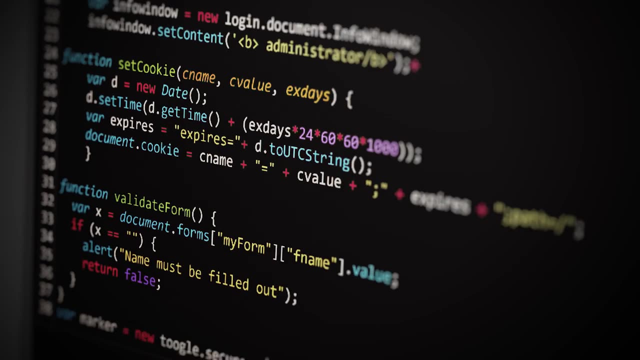 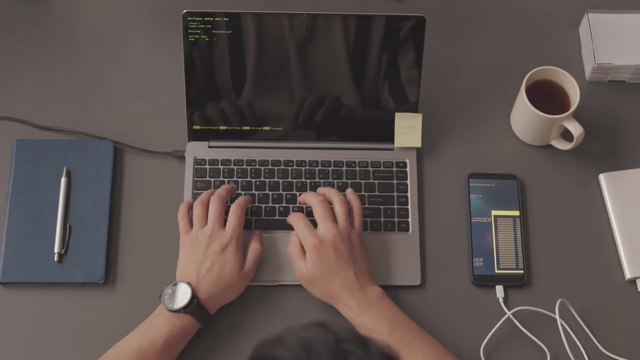 level of versatility you demonstrate, Learn to reverse engineer. The essence of an ethical hacker in any organization is to fortify the system against intrusion. To do that, you need to identify weaknesses in the architecture and reconstruct them such that they can successfully repel attacks. Reverse engineering is a very helpful way to do this. It basically means that 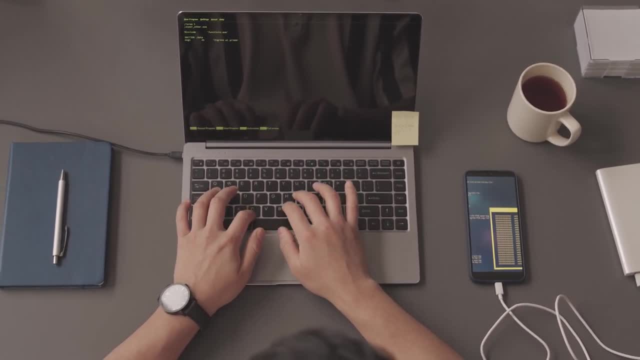 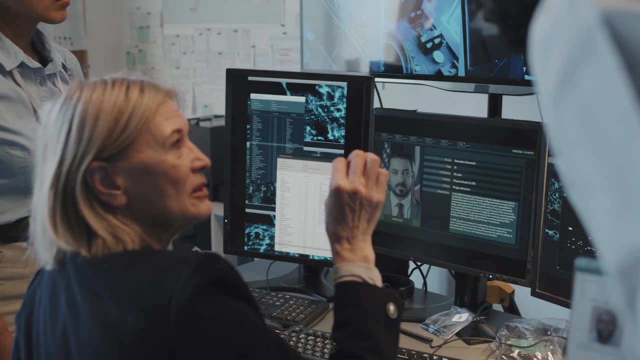 you analyze a product's code and redesign it down to the minutest specifications. This enables you to identify flaws and equip the system against incursions. Database management: Another important part of your job is being able to relate with the organization's systems in a way that helps you to. 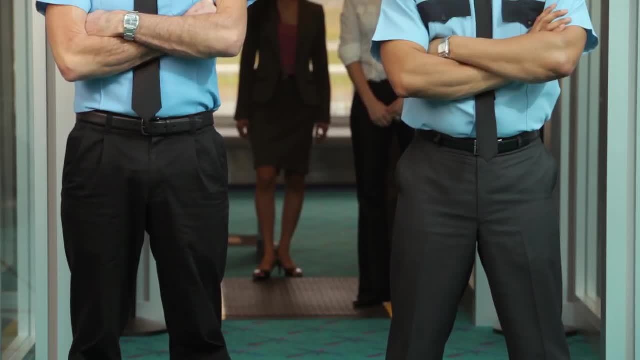 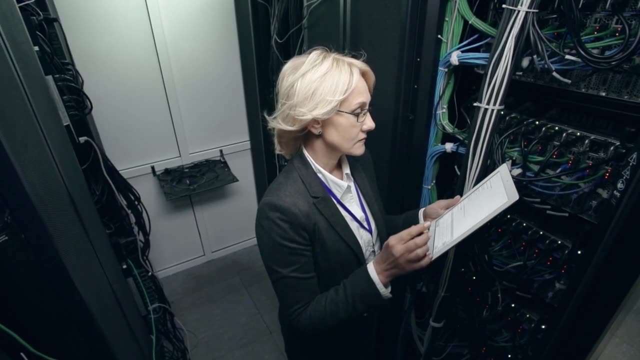 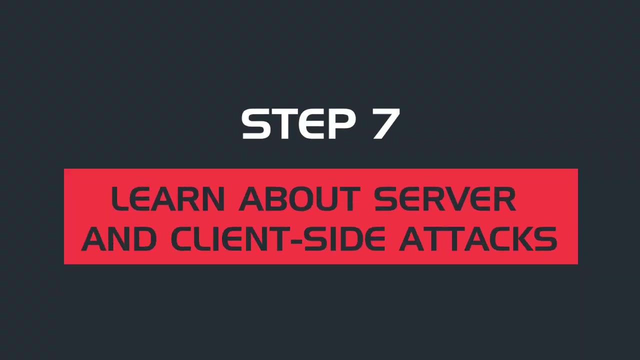 protect them effectively. Like regular security at a physical establishment, you need to know the layout of what you are expected to protect and the interrelationship of different segments. The same applies to database management. Learn about server and client-side attacks. Server-side attacks are designed to compromise. 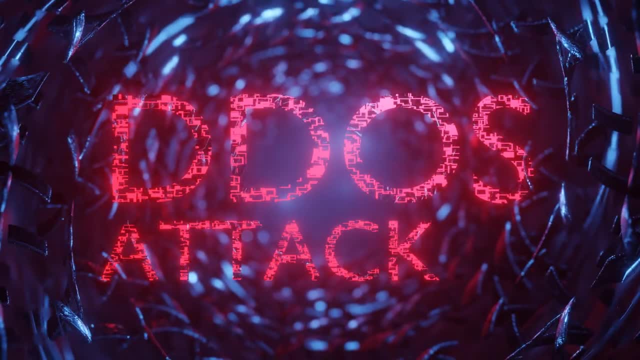 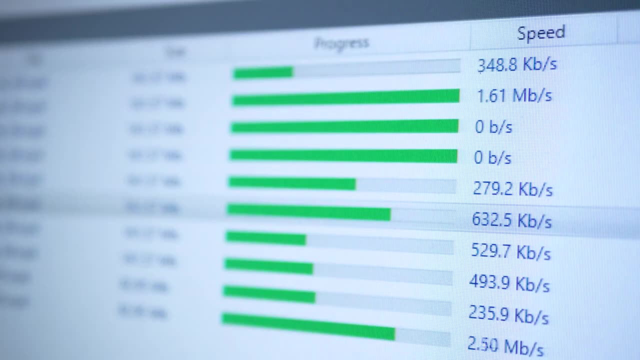 data stored on a target server. They include DDoS attacks, SQL injection and DOS. Client-side attacks, on the other hand, are aimed at software on the device of a client or user. It typically occurs when you unknowingly download malicious software onto your desktop or mobile device. 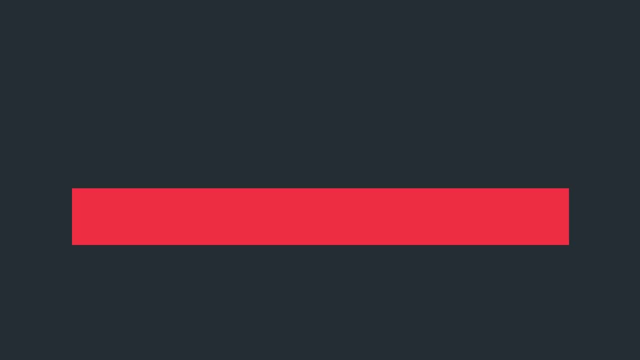 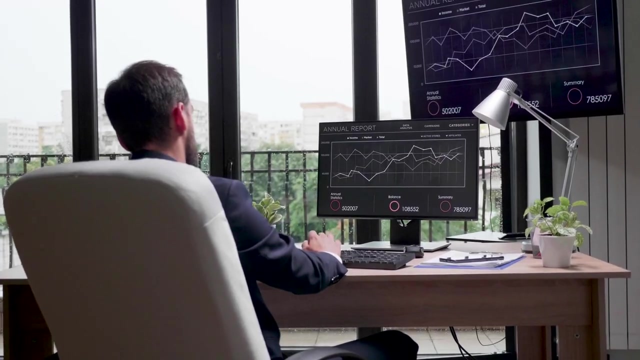 By learning how both work, you can orchestrate one yourself or shield against it. Understand hardware: There are different parts of a computer system. they include your mouse, keyboard, speaker, monitor, etc. To utilize a computer you need to know how these parts work and their specific functions In the process of man-to-machine. 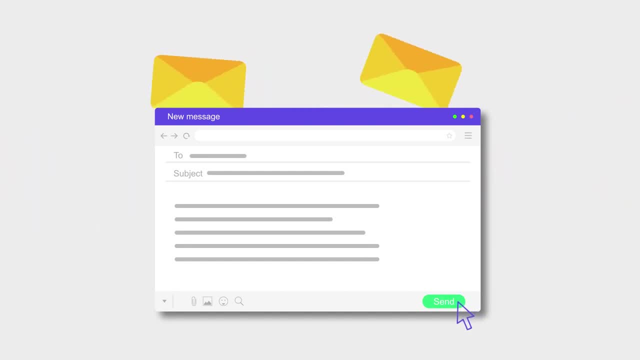 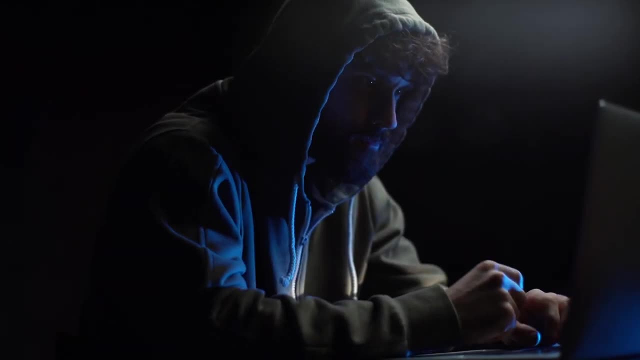 communication. this way, you can deliver accurately to a network the exact functions you want it to embody: Information gathering. A hacker's job is incomplete if he does not understand the rudiments of collecting information. Remember that being an ethical hacker does not translate to not doing. 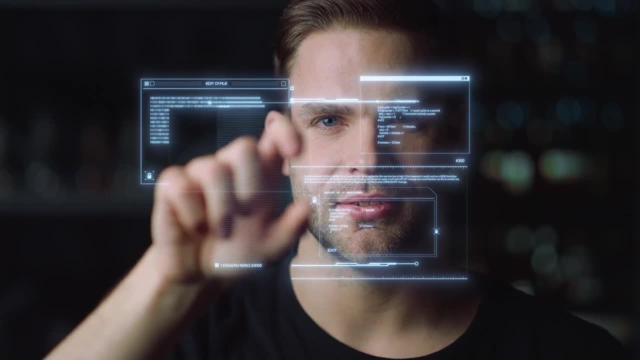 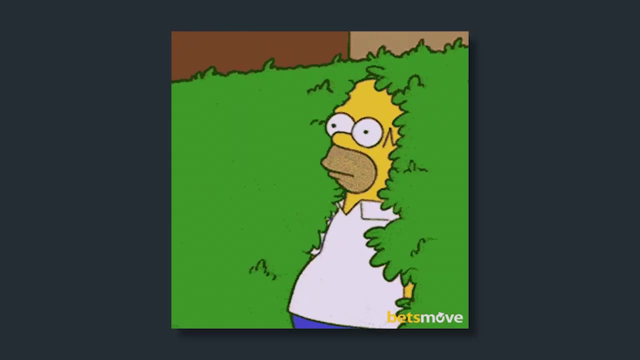 what black hatters will normally do. You must be able to collect information on various internet platforms in the same way to understand how they might be exploited In an attack run. Hone your skills in entry and exit techniques, leveraging tools like Unicorn Scan. 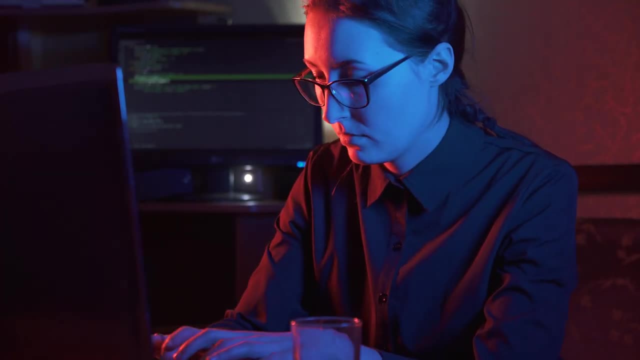 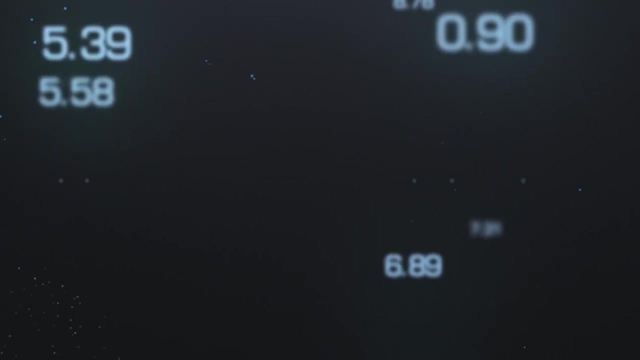 Nmap Dig and your value as a white hat will exponentially increase Cryptography. If you want to prevent sensitive data from landing in the hands of a third party, you need to secure such information by encrypting it so that, even when it is accessed. 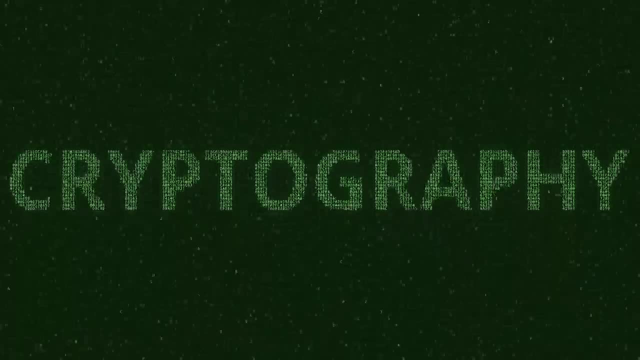 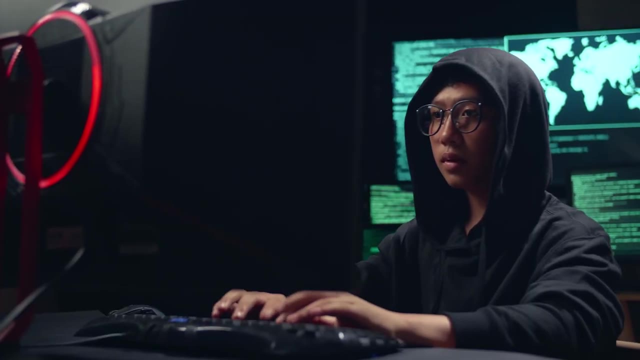 it makes no sense to an intruder and cannot be utilized. Cryptography is concerned with the techniques used in obscuring the true meaning of data. It revolves around the idea of information security and will be required for forcing malicious hackers to watch your data. 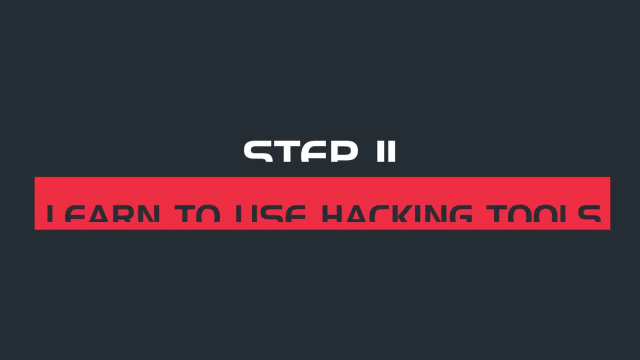 Cryptography is concerned with the techniques used in obscuring the true meaning of data. It revolves around the idea of information security and will be required for forcing malicious hackers to watch your data. Why are they even bothered in the first place? Learn to use hacking tools. Finally, as a hacker, you need to be up to date on changes within the 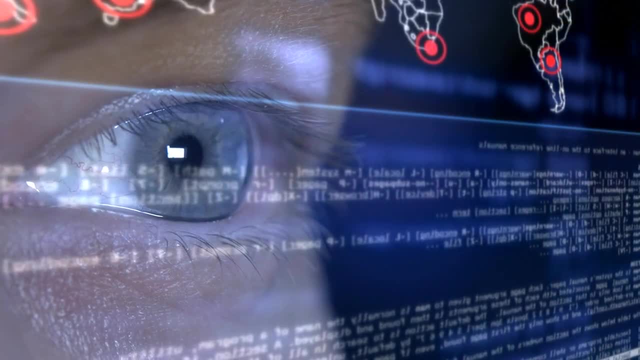 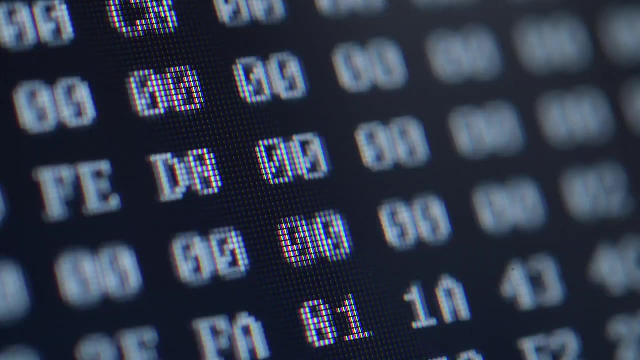 industry. What tools are being developed? The latest techniques that malicious hackers use On the tools end. familiarize with Metasploit, which eases the entire process of breaching a system. Jack the Ripper for cracking user passwords. BEF, for launching sophisticated 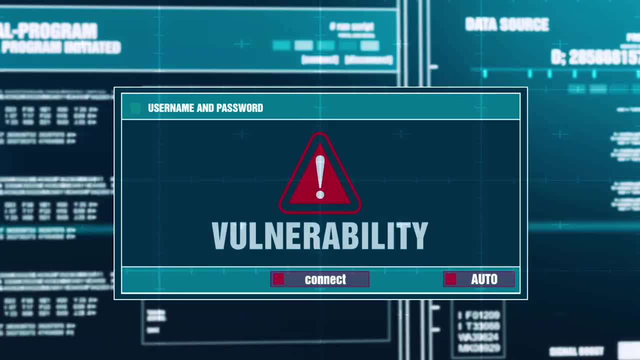 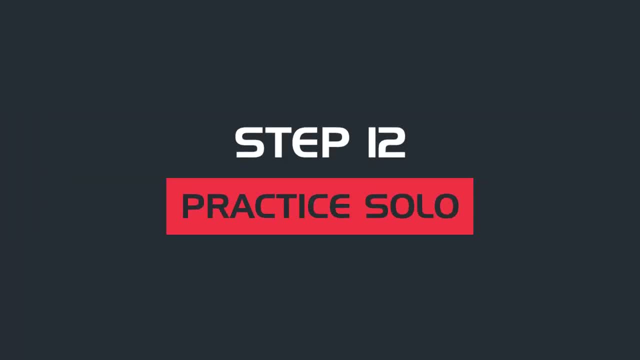 attacks on web browsers, Burp Suite for vulnerability tests and a bunch of others. By the way, let us know in the comments which other tools are interesting and we will add them in the description later. Solo, Much of your actual expertise will come from the efforts you apply yourself, Earlier.